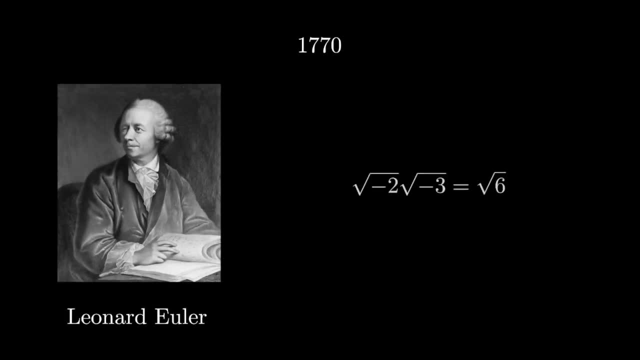 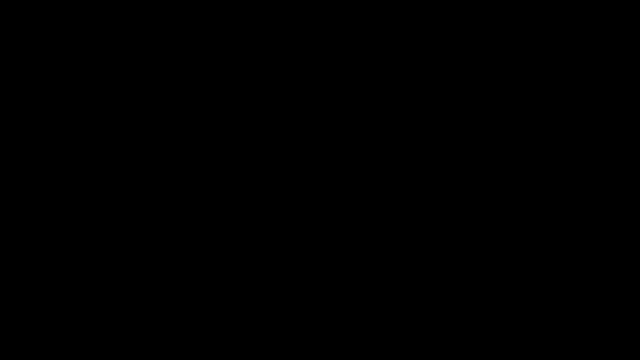 for a great Euler to argue that root of minus two times root minus three is equal to root six. There was no satisfactory answer to the question: what is a complex number which frightened mathematicians throughout generations? A first satisfactory answer to it only came in the end of 18th century from Wessel. 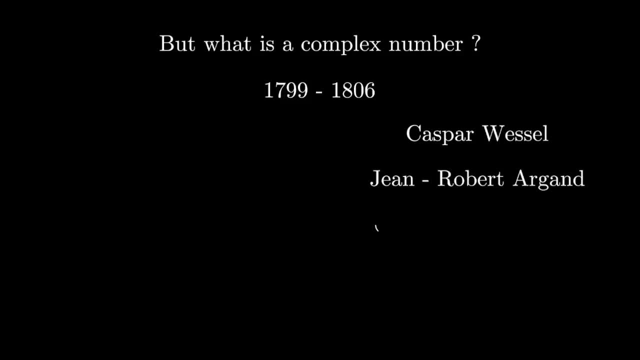 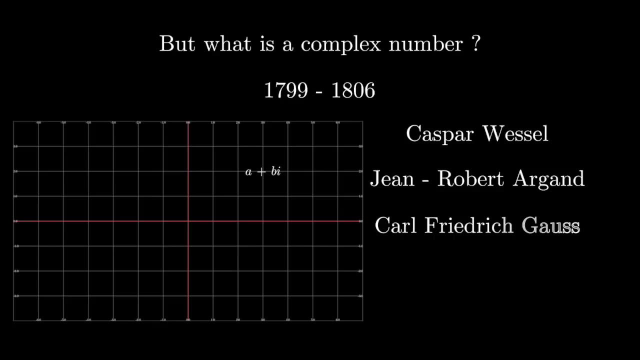 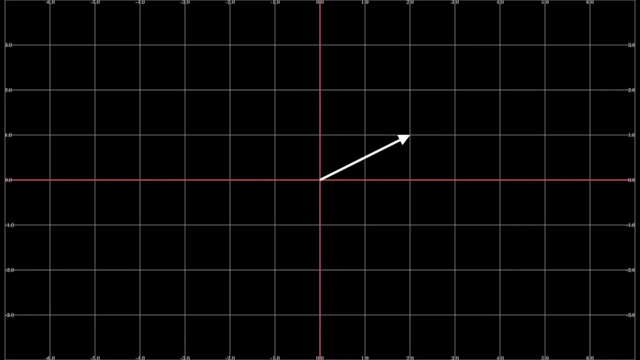 Argand and Gauss, who introduced the visual representation of a complex number independently from each other. They said that you can view a plus bi simply as a point on a two-dimensional plane. These vectors obeyed a normal vector addition rule, but the multiplication rule was weird. 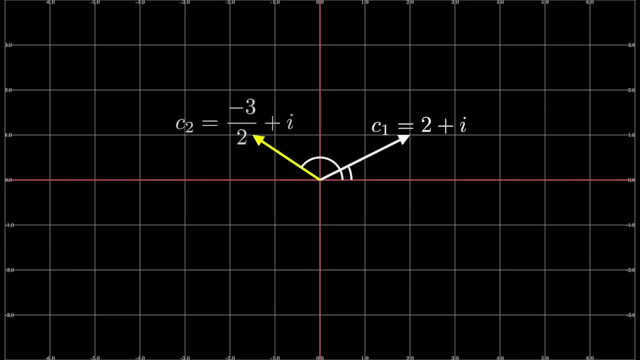 Multiplying two complex numbers is equivalent to adding the angles they make with positive real direction and multiplying their length, which you calculate using Pythagoras. This rule is not obvious, but you can at least see that it is consistent with our expectations. Three i is three times i. 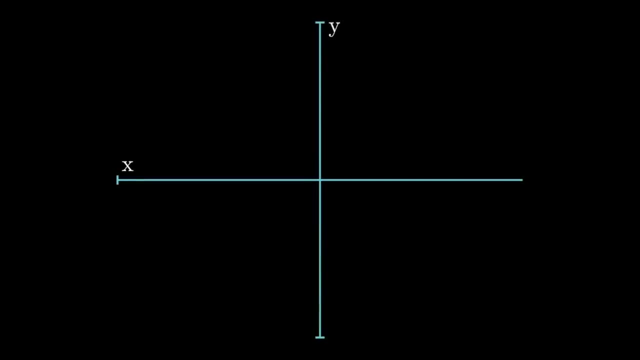 Mathematical traditions in the 16th and 17th centuries were still heavily influenced by ancient Greek mathematics, which was very geometrical. So when someone points out that x squared plus four, x plus five, has a negative discriminant, anyone from 17th century would reply: 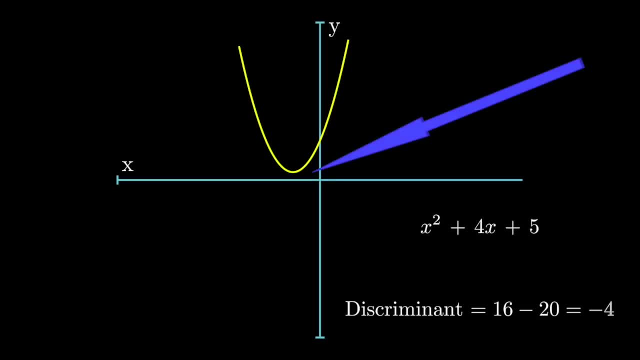 well, this parabola does not intersect the x-axis, so we will discard this case as useless. Once again, the quadratic formula was not sufficient for overcoming the psychological discomfort of introducing complex numerals. Surprisingly, it was a cubic equation which broke the barrier. 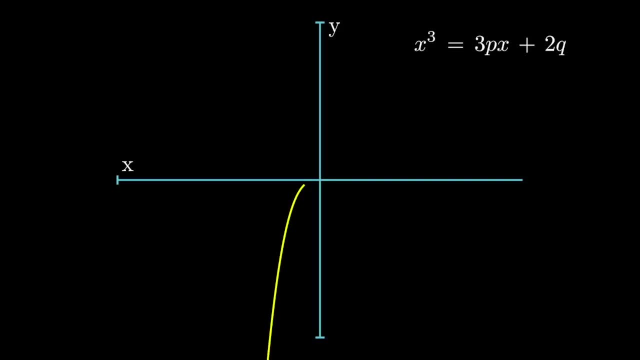 This equation is basically saying that we need to find all points of intersection of a cubic and a line: 3px plus 2q. Cardano produced a remarkable formula for finding the root of this equation. 30 years after this result, Bembelli encountered something strange. Look at this example: Here p is 5 and q is 2,.